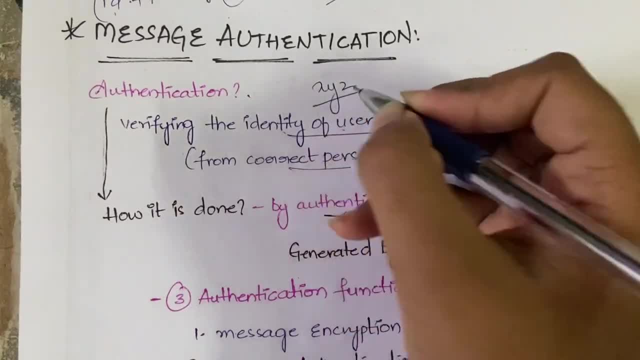 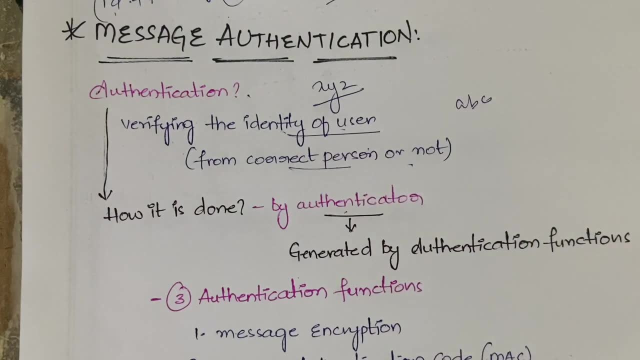 in an organization. some XYZ organization got it. If somebody from other organization- let us take like ABC organization- wants to come and access to your data, will you give the data to him? know, right, we will be having some security, we will be having some confidential. 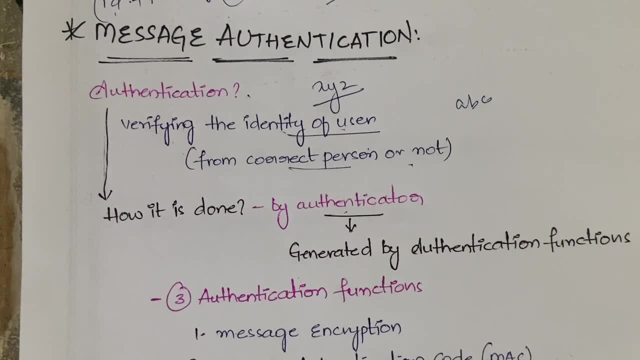 data which we have to not share with others. So that is why first it will check whether the, whether the mail or whether the request or whatever it is, it is from the correct person or not. suppose, see, if you're when you're working, you'll be getting. 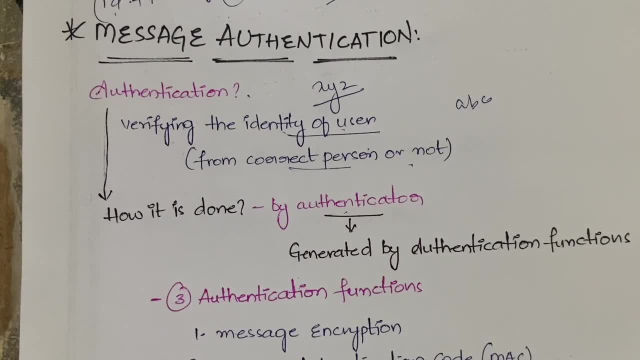 a email id from your company- outlook id- right, so it will end with some domain name. so if somebody from other domain will come, or if somebody from other domain messages you or request you for the data, you'll not give them right. so that is what authentication is: whether the person is correct. 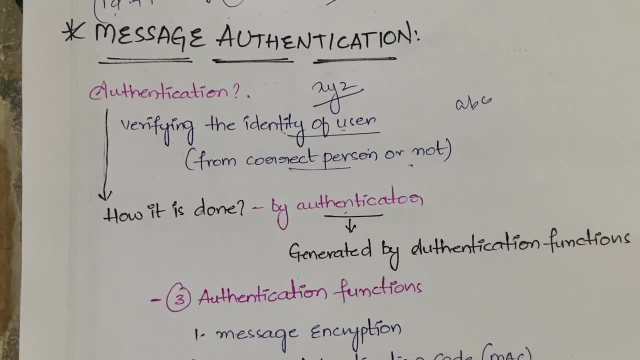 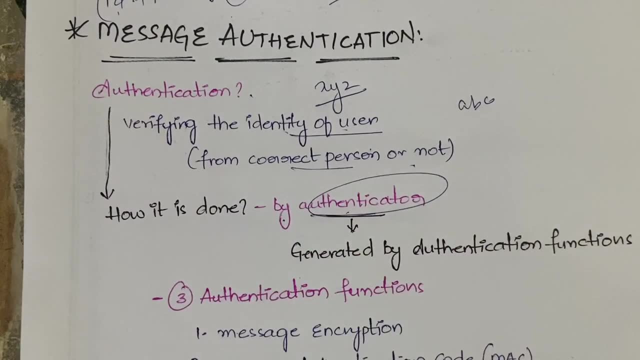 or not. whether we have, we can share data with that person or not. that is authentication. and how do we do the authentication? we do it with the help of the authenticator. got it? so what is this authenticator? it can be a number, it can be a hash code, it can be a function or it can be. 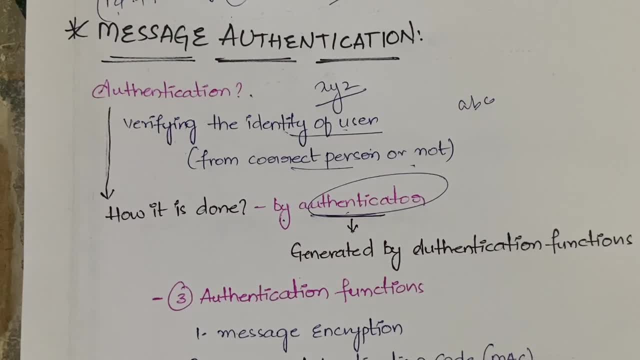 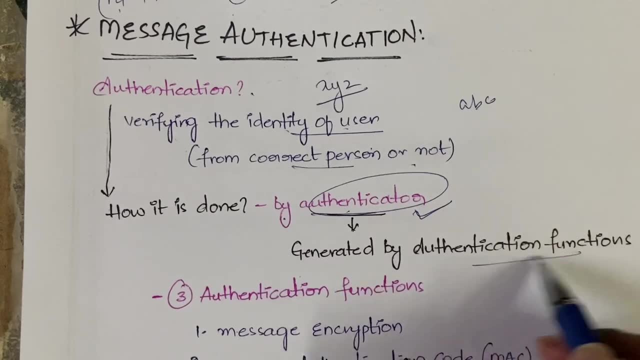 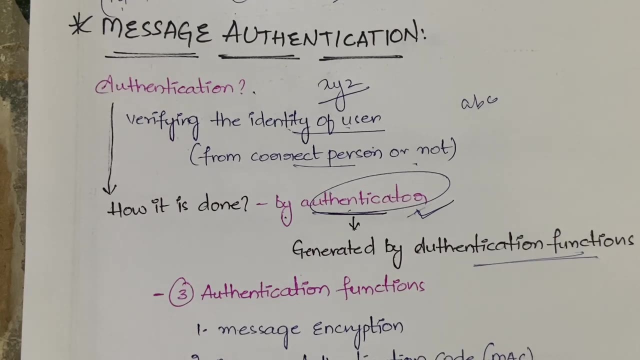 alphabetic and alphanumeric. whatever it is, it can be anything. and how do we get this authenticator? it is generated by authentication functions. with the help of authentication functions, we will be generating, the authenticator got it. so now we have different types of authentications. we actually authentication function. we have three. 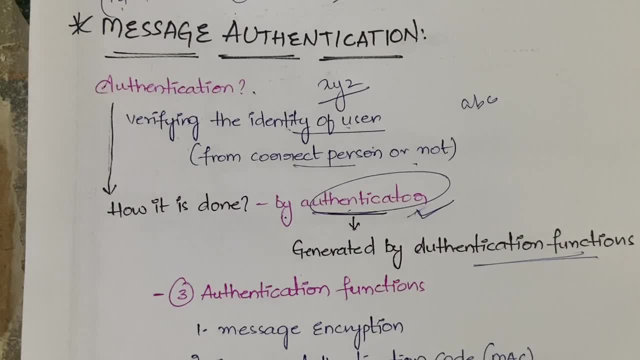 so we have three authentication functions. we have three authentication functions. we have- let us see them now also, and some of them i will be explaining you in detail- which is required, like if anything is, detailed description is required for anything. i'll definitely give you that as well, right? so what are the three functions we have for authentication? they are message. 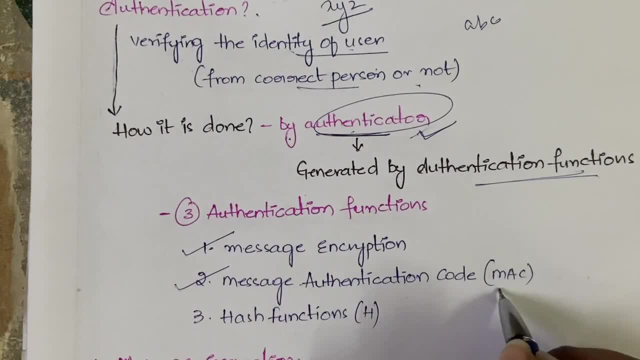 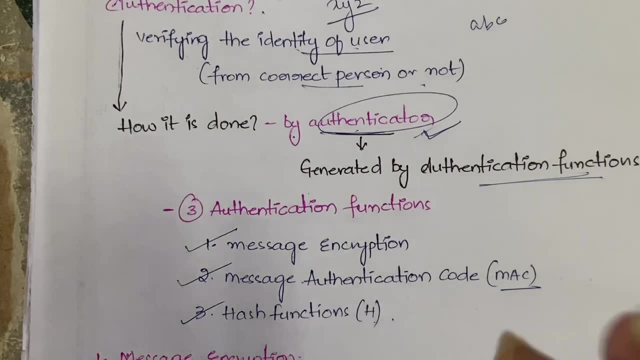 encryption message, authentication code, which is, in short, called as mac, mac, okay. and third is hash functions, denoted by capital h. got it. so we have three authentication functions in order to generate the authentication code. so we have three authentication functions in order to generate the authentication code. 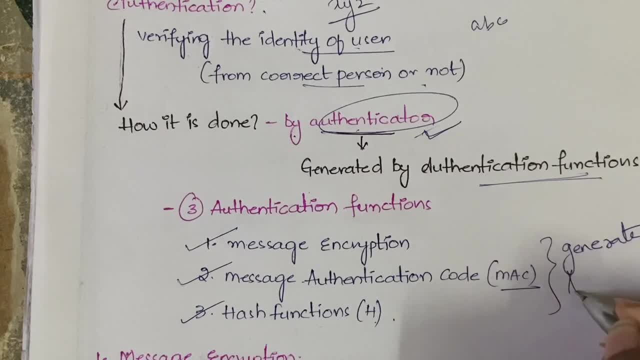 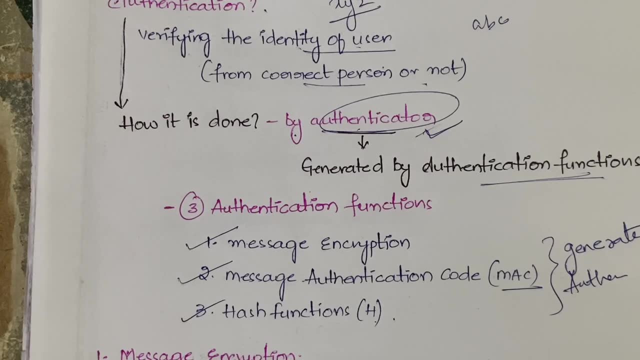 real computer and literally the trzy引ńsk length. even if i go inside the进ฯ, i go. let me do the same thing: números dosing. now, these three ones mean um methods, and then this one are toเรา got it. now, what are those three? message encryption message. author: Railcode. 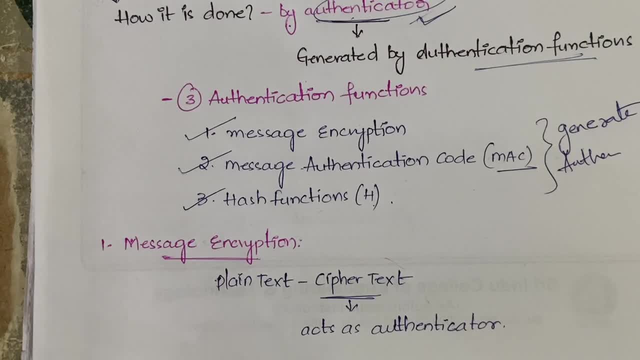 which is nothing but Mac and hash functions denoted by hatch. got it now. so let us see about message encryption first. so you know what encryption is very common thing. encryption means right. so that is what message encryption means. and here, which will act as authenticator? the ciphertext which is generated will act as your authenticator. 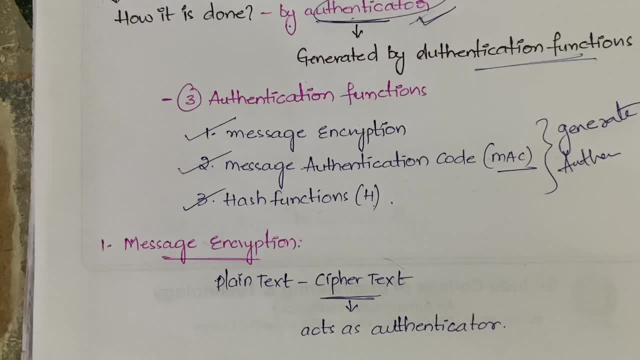 got it. so this is about message encryption very simple. the process of conversion of plaintext to ciphertext is encryption that we already know, and in this process, we will be using keys, we will be using a network, we will be using some encryption algorithms as well and in this situation, ciphertext, which is 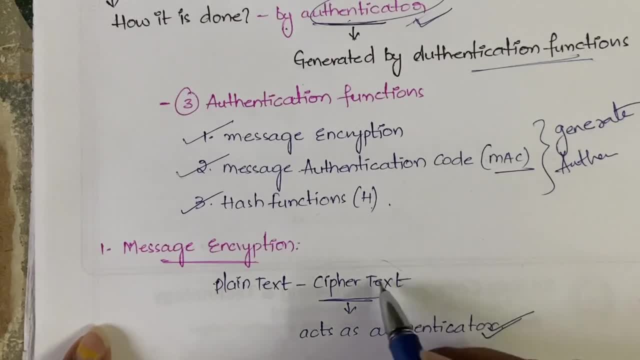 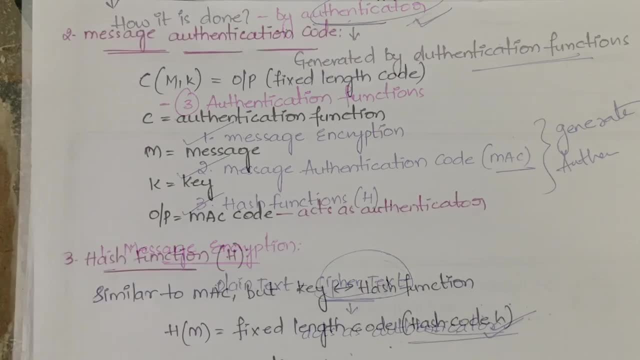 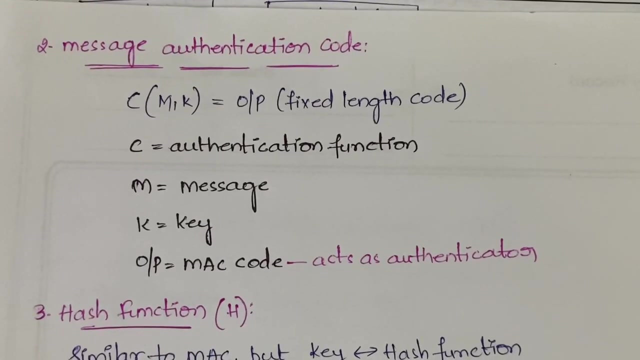 generated will be acting as the authenticator. with the help of this ciphertext, we will be checking the authenticity. got it? so now let us see the next one, message authentication code. so in message authentication code, this is also very simple. so C of M, comma K is equal to output. so what is this C? what? 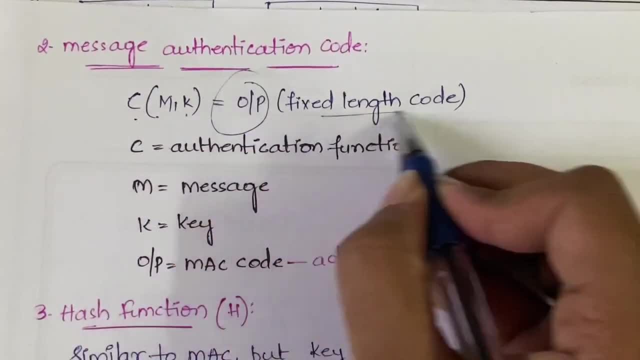 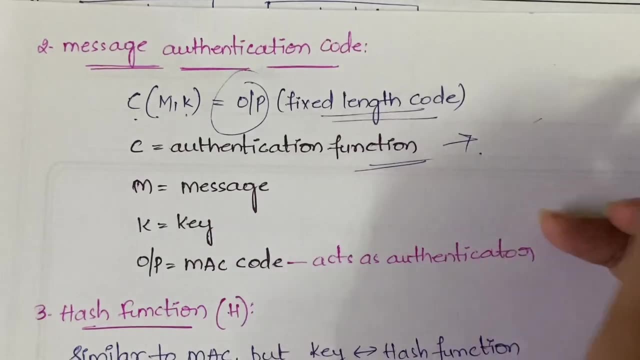 is this capital, M, K, I'll tell you. and this output which you get will be your fixed length. okay, so here, C is nothing but the authentication function. with the help of this, we will be generating the authenticator, right? so C is the authentication function, and and. 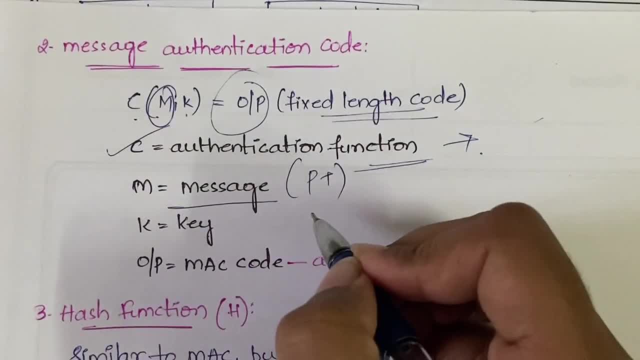 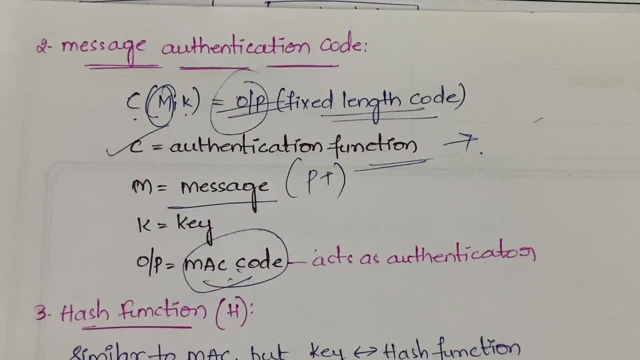 M stands for message, which is nothing but the plaintext. also, you can say: and K stands for key and output stands for the MAC code. MAC code is nothing but the output which you get. it is a fixed length and this MAC code will act as the authenticator, like how ciphertext in case of message encryption. this was the 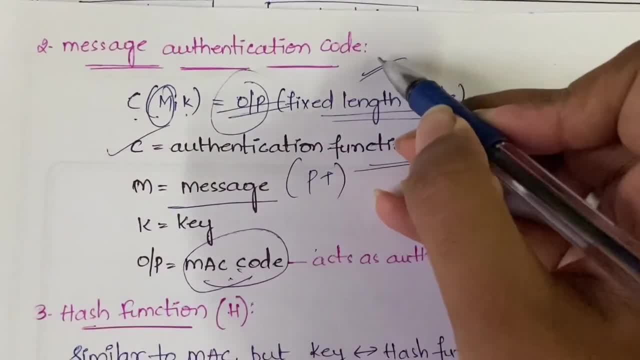 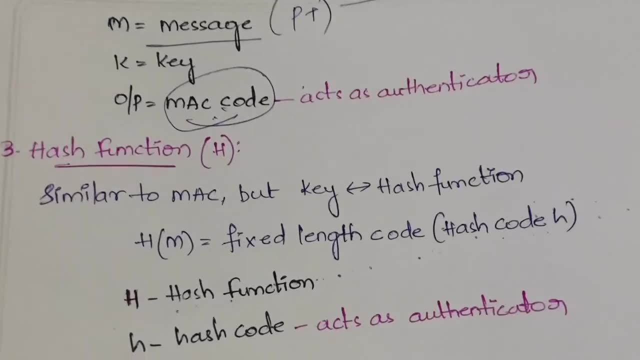 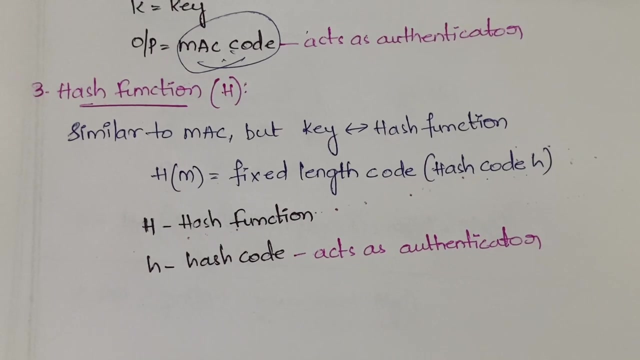 same MAC code will act as a authenticator. in case of MAC got it, message authentication code got it. so this is about. next, we have hash function, which is denoted with capital H. this is also very much similar to Mac, but here, in case of key, you will be using the hash. 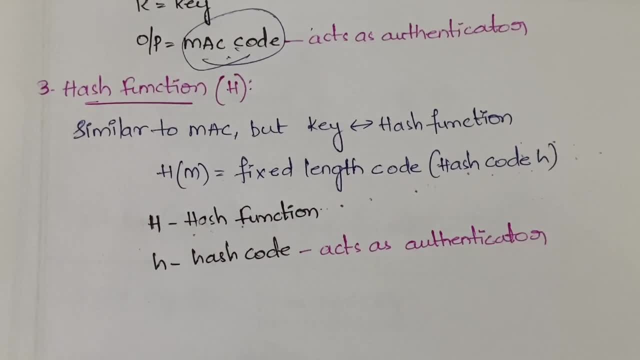 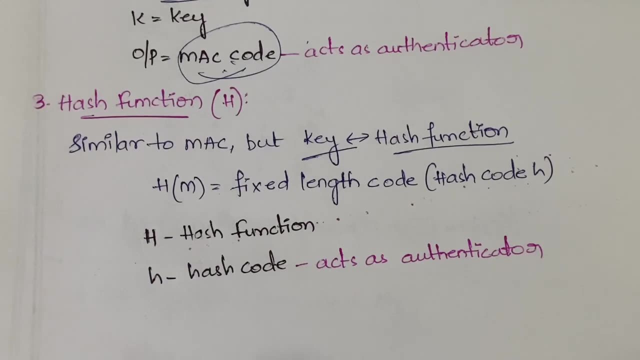 function. got it. in place of key you will be using the hash Ready hash function. key is replaced with hash function, got it so? if you can see here, H of M is equal to again, fixed length code. you will be getting which is nothing but the hash code, and this hash code is denoted with small H, Capital H.